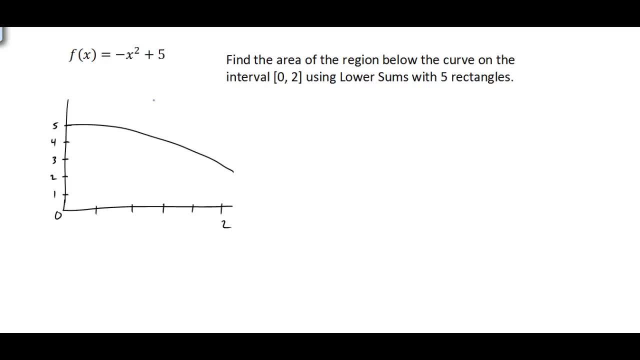 So they want us to use 5 rectangles to estimate the area that's underneath this curve on the interval from 0 to 2.. So first of all, we need to calculate what is going to be the area that's underneath this curve. So, first of all, we need to calculate what is going to be the area that's underneath this curve on the interval from 0 to 2.. 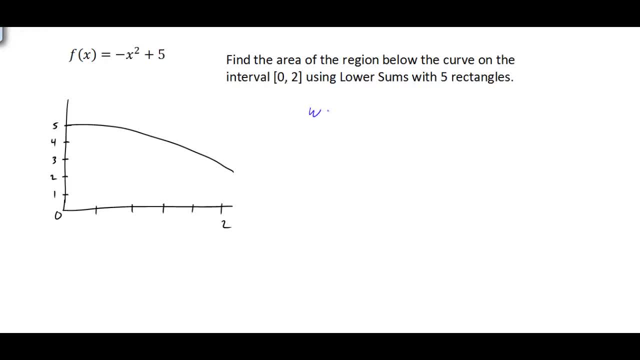 So, first of all, we need to calculate what is going to be the area that's underneath this curve on the interval from 0 to 2.. So, first of all, we need to calculate what is going to be the area that's underneath this curve on the interval from 0 to 2.. 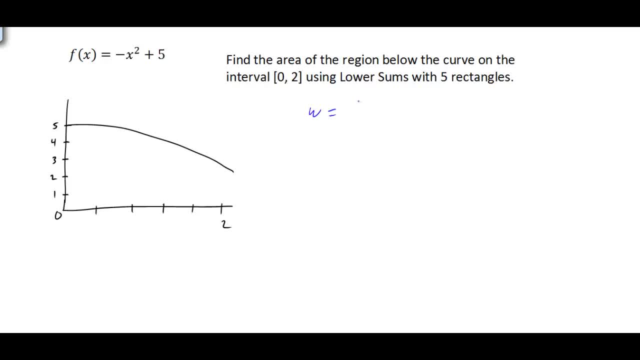 So, first of all, we need to calculate what is going to be the area that's underneath this curve on the interval from 0 to 2.. So, first of all, we need to calculate what is going to be the area that's underneath this curve on the interval from 0 to 2.. 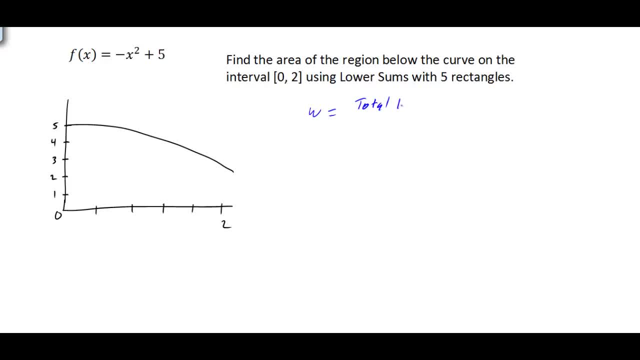 So, first of all, we need to calculate what is going to be the area that's underneath this curve on the interval from 0 to 2.. So, first of all, we need to calculate what is going to be the area that's underneath this curve on the interval from 0 to 2.. 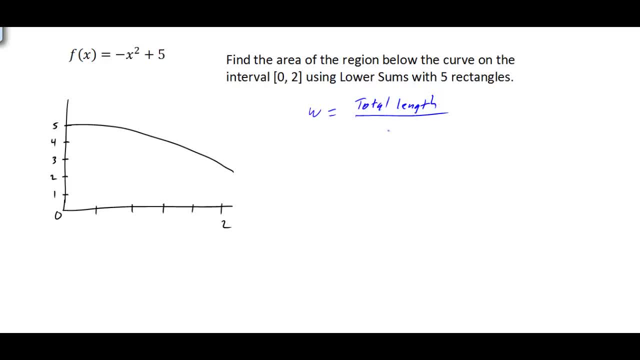 So first of all, we need to calculate what is going to be the area that's underneath this curve on the interval from 0 to 2. divided by the number of rectangles that we want. so in this case, if our intervals from 0 to 2, we 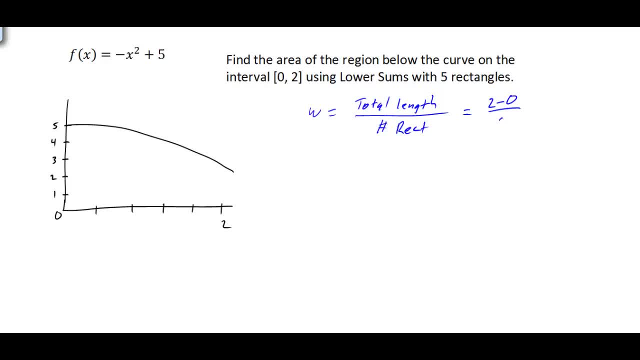 could simply take 2 minus 0 divided by the number of rectangles. so therefore we're going to use a width of 2 fifths. so we need to mark off each rectangle on the axis here. so if we start with 0, we're going to add 2 fifths. 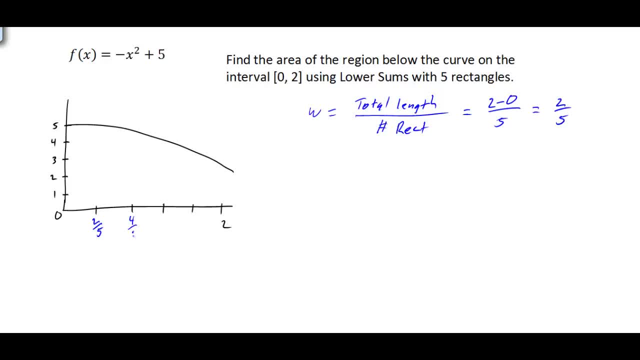 and then we would get 4 fifths, 6 fifths, 8 fifths, and then, of course, we would end up here with 10 fifths, which would be equal to 2. so now we have our markings for our rectangles. so, in other words, we're going to start and we would have 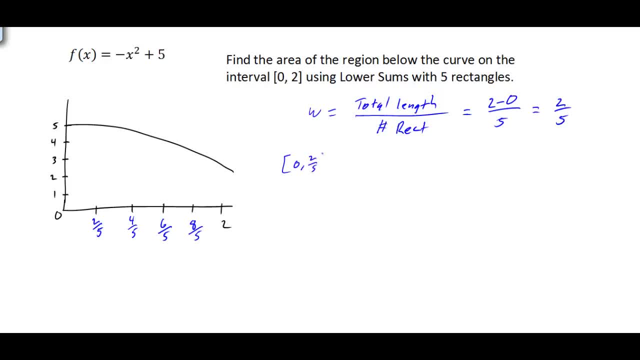 first rectangle would go from 0 to 2 fifths. our second one would go from 2 fifths to 4 fifths, and so on. so I'm going to mark off each of our rectangles, alright? so here we have the left and right endpoints of our rectangle. 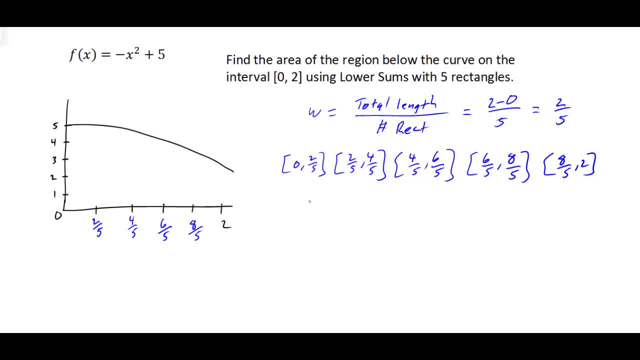 now, because we're looking at the lower sums, we're looking at drawing our rectangles below the curve. so with this problem, if you notice, if we were to draw up from 0 and over, we're going to go above. but if I start from 2 fifths and if I go, 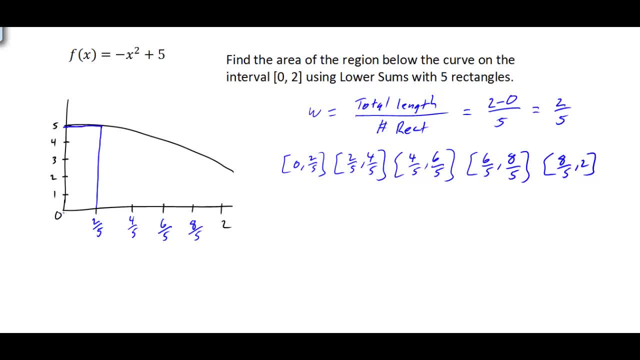 up and then over to 0. so therefore, notice, our rectangle is below our curve, and then we could draw. we go up at 4 fifths and then at 6 fifths, and then at 8 fifths, and then at 2, 0, and then at 8 fifths and at 2, so you'll notice that our area here is going to be a little bit less. 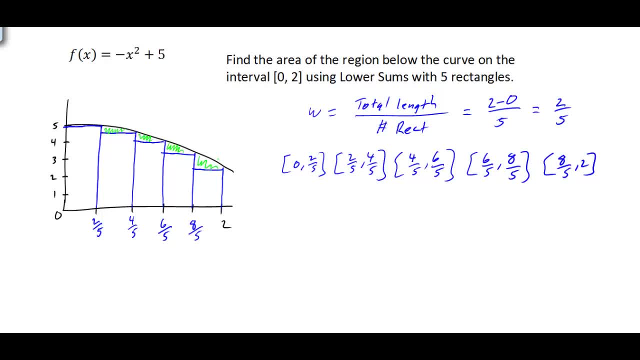 because we're missing this part here. so the question is: if we look at this closely, notice we're going to calculate the area of each rectangle. so if we look at the first rectangle here goes from zero to two-fifths, so we know that the width is two-fifths. So if we're looking at the area, we 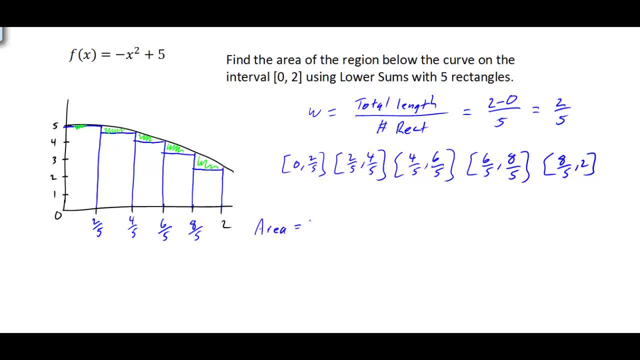 could simply say: the area is going to be equal to the width of two-fifths, and then we need to find the length of the first rectangle. So here we have rectangle number one. Now do we want to use the left side of the rectangle at zero, or do we want to use the right side? And you're probably thinking. 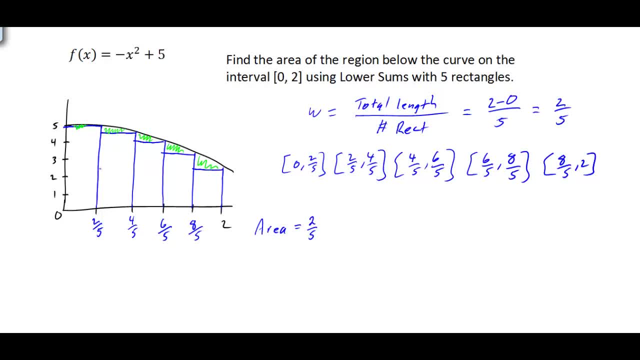 does it really matter? Well, for this problem, notice, the only way we can find the length, which we'll call this l1 for this first rectangle, is if we go all the way up. Notice the right side of the rectangle and this is the important part: to understand The right side of this rectangle. 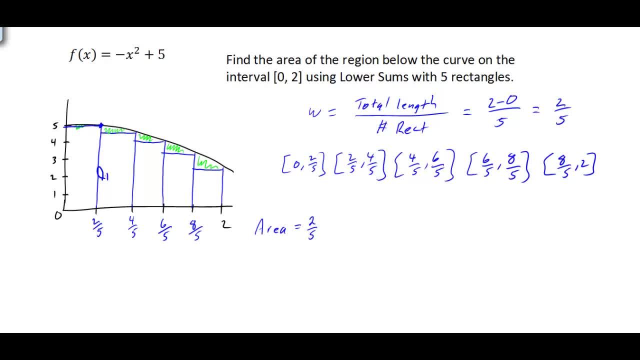 when it goes up it touches the graph. at this point here The left side doesn't touch the graph. So we know we can find l1, because that's just simply what. That's simply going to be the y value evaluated at two-fifths. So if you go up to the graph, we could go over to find the y value or in: 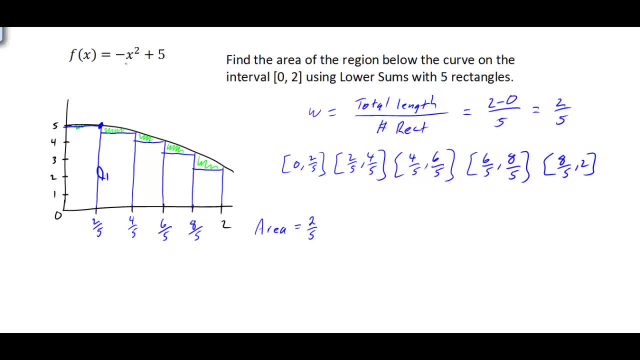 other words, we could take two-fifths and plug it into the function above: negative x squared plus five, and that will give us l1.. So we need to take two-fifths times l1 plus two-fifths multiplied by l2.. Well, that's going to be our second length here And again, notice this. 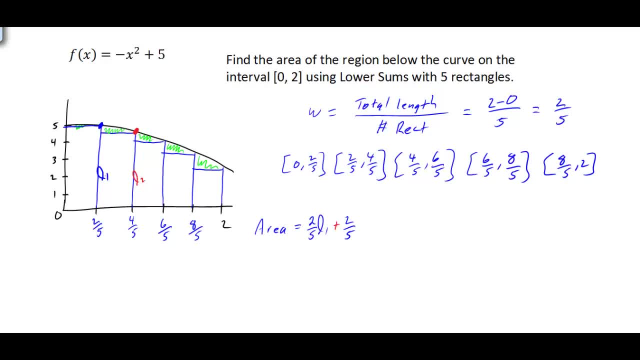 right end point of two-fifths touches the graph. And then we would have two-fifths times l2 plus two-fifths times l3. And notice that's going to touch the top of the graph here, Plus two-fifths times l4.. And notice, here again, this point touches the graph here. So we use the right. 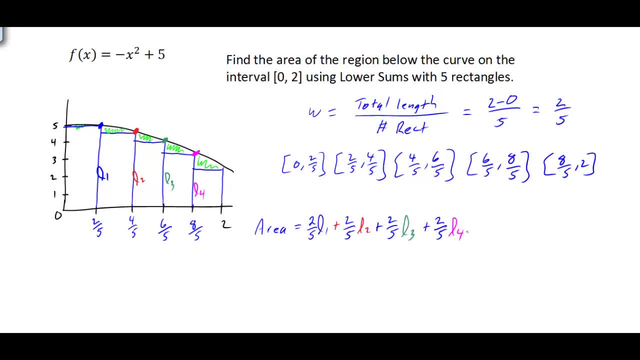 So that's two-fifths times l4 plus two-fifths times l5.. So, if you notice, we're using the right side of our rectangles to calculate the length. Now to make things a little bit easier here, Notice, here each one of these is: 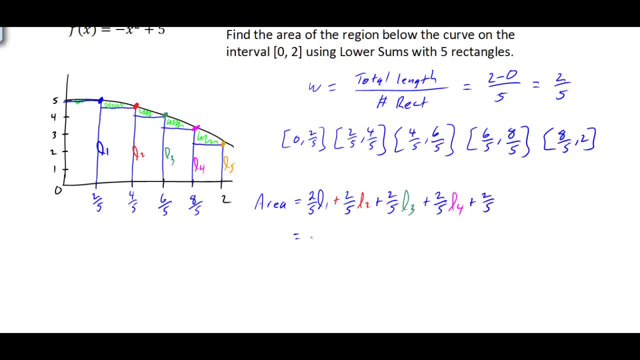 multiplied by two-fifths. So we could simplify this by simply factoring out the two-fifths so that we do not have to write this over and over. So we would simply have l1 plus l2 plus l3 plus l4 and plus l5.. 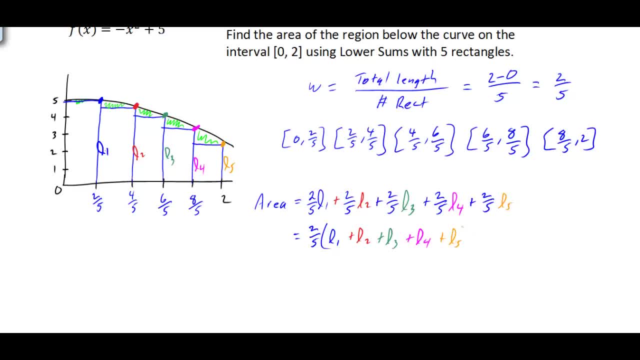 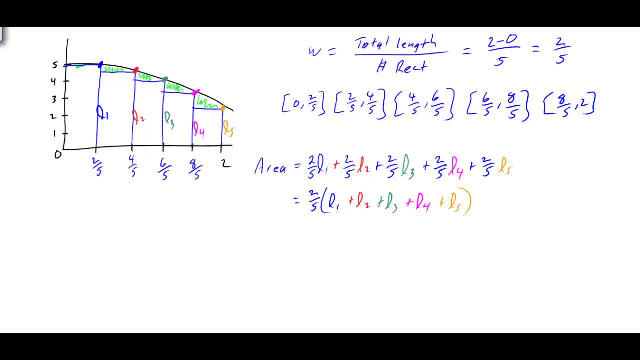 L5, so that way we don't have to multiply the two fifths, we can just do that at one time at the end. so now, how do we actually find this L1? well, L1 again, we're looking at the two fifths, so we're simply going to plug that two fifths, like I said before, into the original. 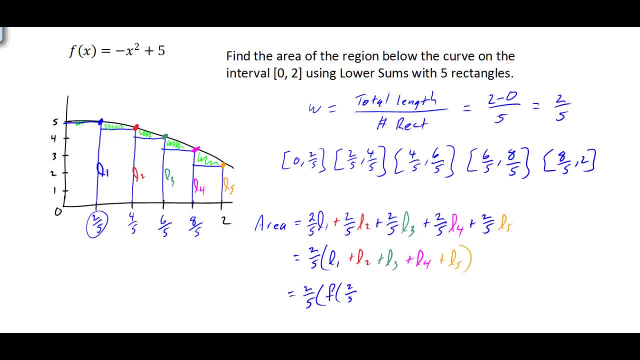 function negative x squared plus five. so we want to evaluate two fifths. I'm sorry, we want to evaluate the function at two fifths. and then we want to do the same thing for L2, except for here, this is going to be evaluated at four fifths. and then for L4- whoops skipped L3. for L3, we're going. 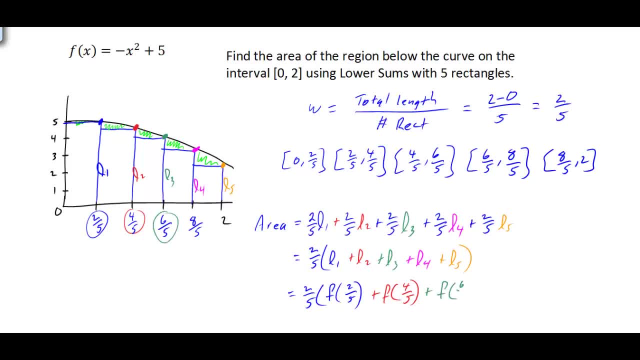 to use six fifths, and then for L4 we have eight fifths and L5 f of two. so now, this is the part we don't want to forget. we want to take actually each one of these. now, of course, this means your function f is evaluated two fifths, so we're going to plug. 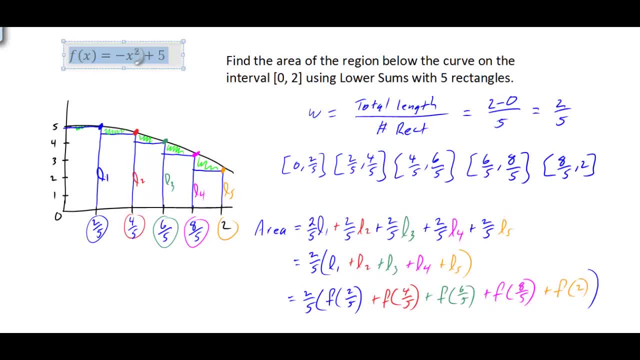 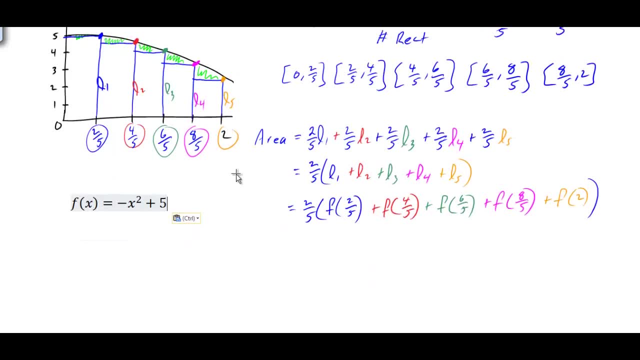 that into this function f of two. so we're going to plug that into this function f of two. so we're function here. so if we're going to do that here, we would end up with our two fifths out front and then F of two fifths if you plug two fifths into this. 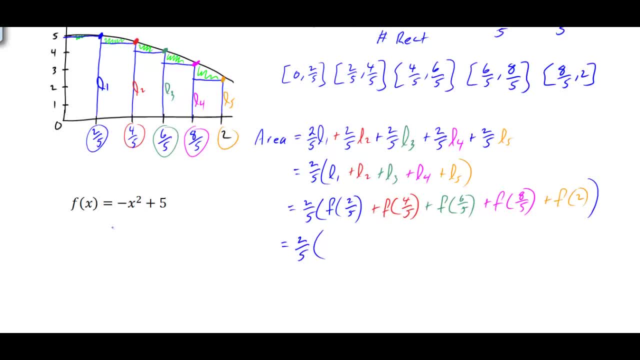 function you're going to get, and keep in mind this would be negative two fifths squared. so you don't want to square the negative, so it's negative. two fifths squared plus five. so you're squaring to two fifths, then the negative, and you're. 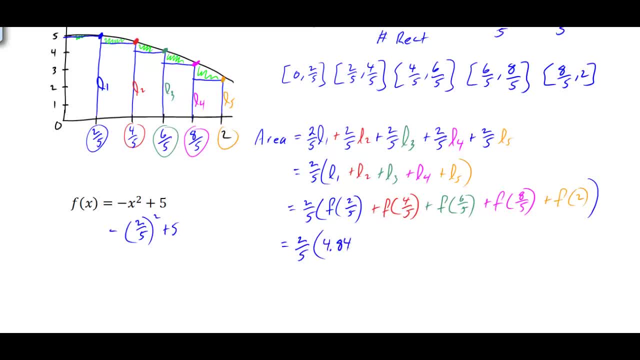 going to end up with approximately four point eight, four, and then we're going to take four fifths and plug that in for X and we'll get four point three, six, and the same thing for six fifths, and we get three point five, six, and if you plug eight fifths into the function, we get two point four, four and 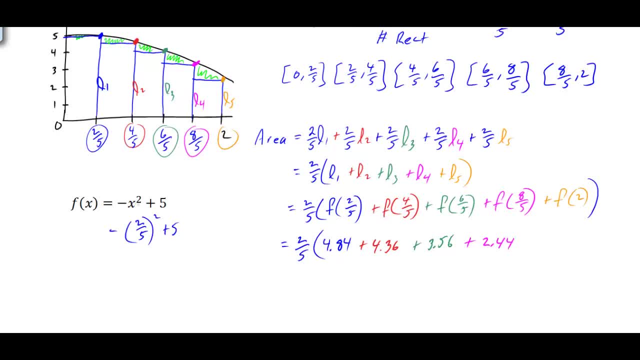 if we plug in two clear, you're going to get four. so it's a negative four plus five. so that would simply be plus one. now keep in mind these values here: four point eight, four, four point three, six, three point five, six, two point four, four and one. that's given us the length here of each of the rectangles: L 1, L, 2, L, 3, L. 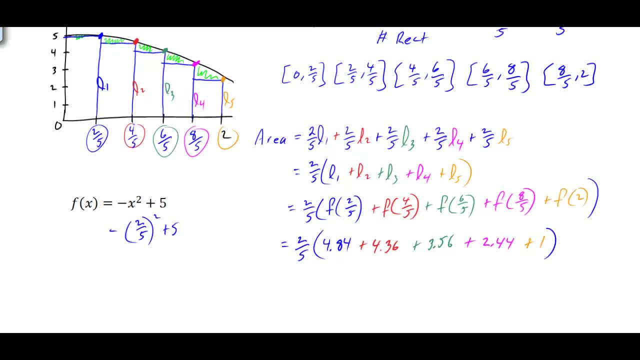 4 and L 5, and that's because if we plug four fifths into the function, that's going to take us all the way up here to this red dot which has given us the height of the rectangle, because it touches the graph at that point, and if 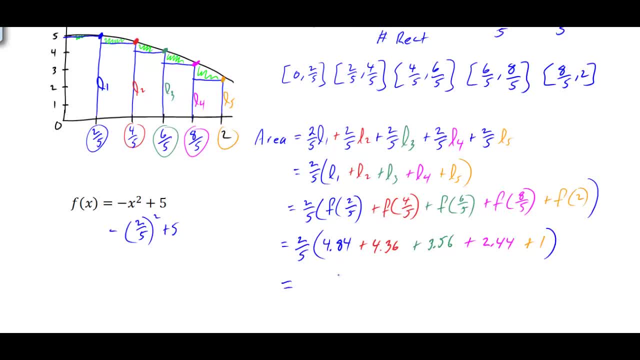 we perform all the calculations here, you're going to end up with an answer of six point four, eight, and keep in mind this is the area that we've come up with and we know this is going to actually be slightly less than the region that we're looking for and that's why we call this the 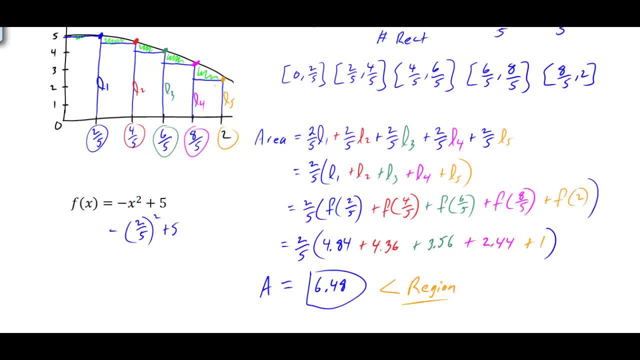 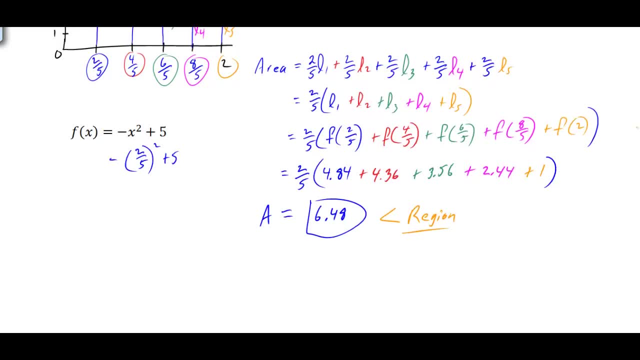 lower sum because it's given us the lower sum or this smaller area for the region. all right, now, quickly, I want to look at how can we use, how could we use the Sigma notation that we talked about before for summation. well, we could set this up. 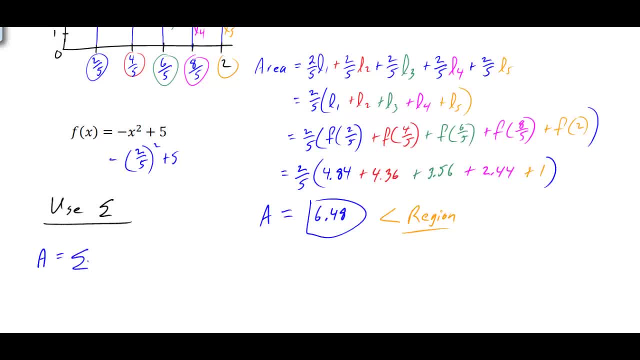 as the area equals, our sum of I equals. well, where we're going to start at? well, we're going to use five rectangles because we want to keep in mind, we want to sum up all five of these rectangles here, so we're going to start at one and 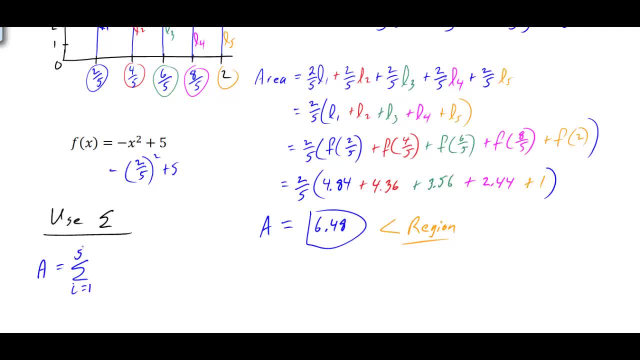 we're going to go to five. now we know the width, just like I factored out over here, our width is always going to be two fifths. so we know that we're going to have two fifths, and now we're going to have two fifths. and now we're going to. 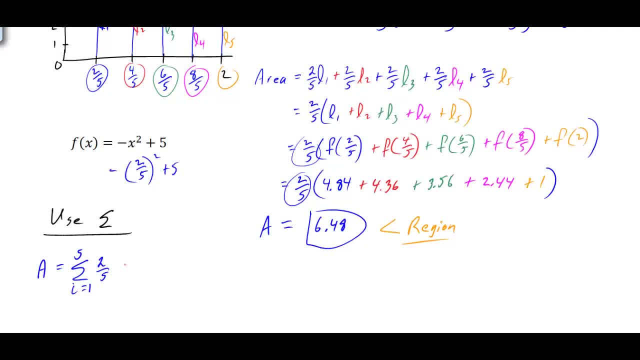 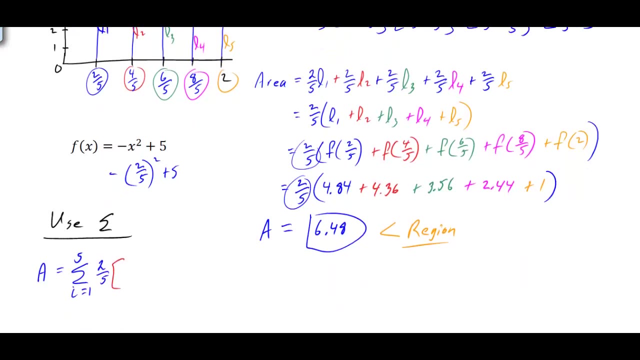 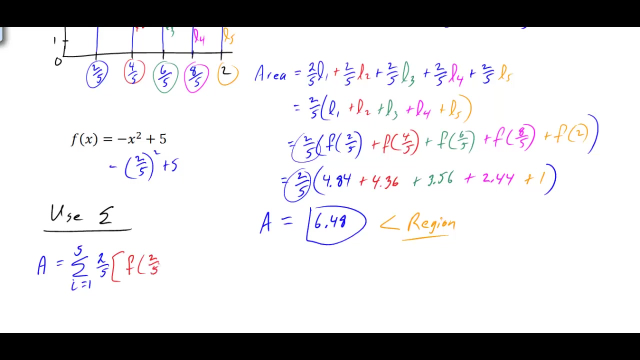 need to figure out. how can we calculate the height? well, we're going to take and plug two fifths. for the first one, we plug two fifths into the function, our first l1, so we could think of f, of two fifths. now, if we plug that into the 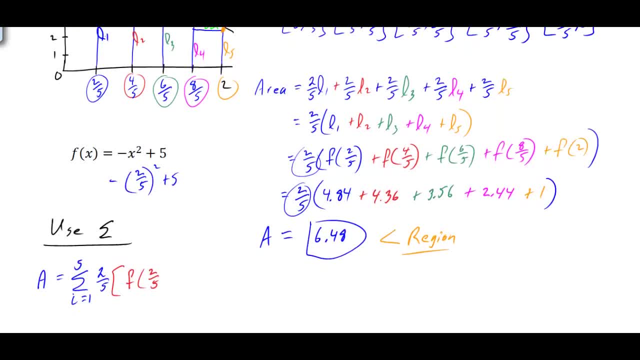 function, that's going to give us the first one. so if we were to plug in, let's say, f of two fifths I, and let's see what happens here: if we plug one in for I, we get f of two fifths and notice over here, that's what we want, right here. well then, 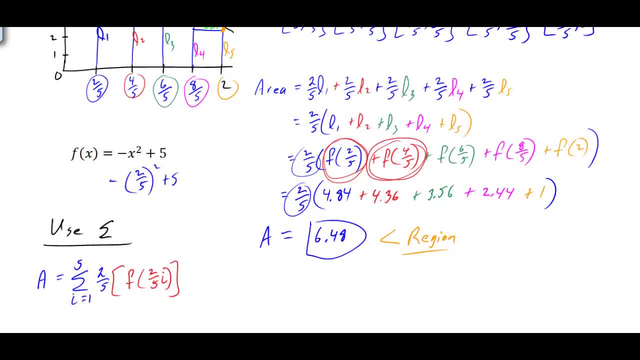 the next one. we want f of four fifths. so when we go from I equals one to I equals two, we plug a two in for I, you're going to get two times two, which is four fifths. so that gives us the f of four fifths. and then we want six fifths. well, 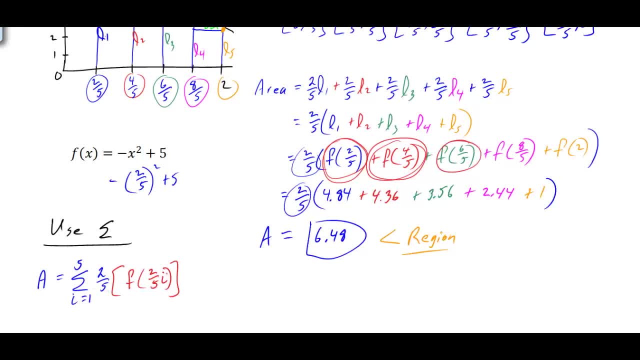 when we go from one to two to three. we plug three in for I, you get six fifths, and if we plug four in for I, we get the eight fifths. so it's f of eight fifths. and if we plug in the five, we get. 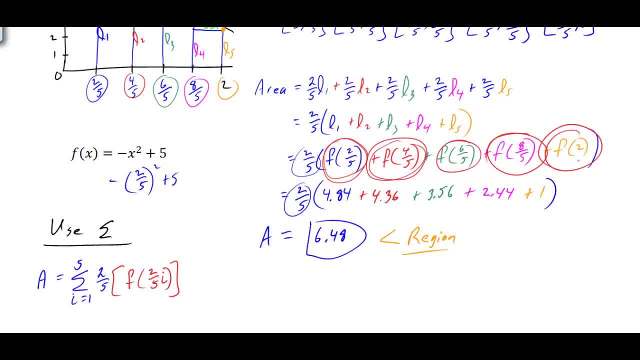 10 fifths, which is the f of two. so this formula- here the two fifths- is giving us the width and the function evaluated at two fifths I. this is going to give us the length of each rectangle and we're going to need to figure out how do we. 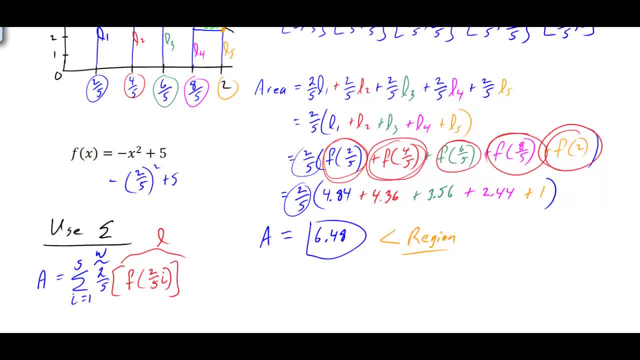 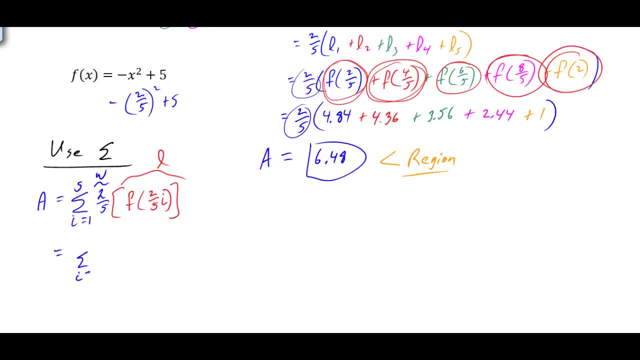 So we want to sum all of these up and that will give you the area. So, for example, we could rewrite this as: the sum of i equals 1 to 5.. Now the two-fifths. you have a couple options. 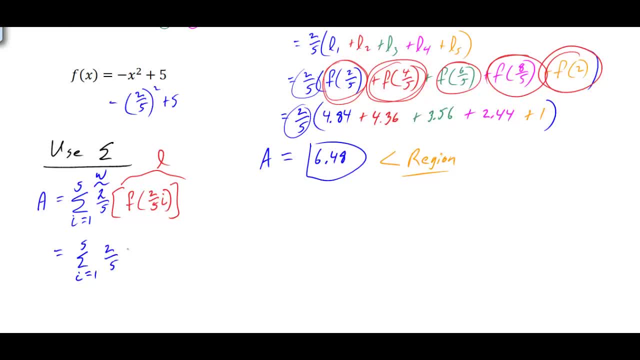 We can leave the two-fifths here, and then we could simply evaluate our function here. Now, at this point, we want to take this whole two-fifths i and substitute this in for the x. Okay, so be careful. So we would have minus two-fifths i and that whole quantity because of the function here. 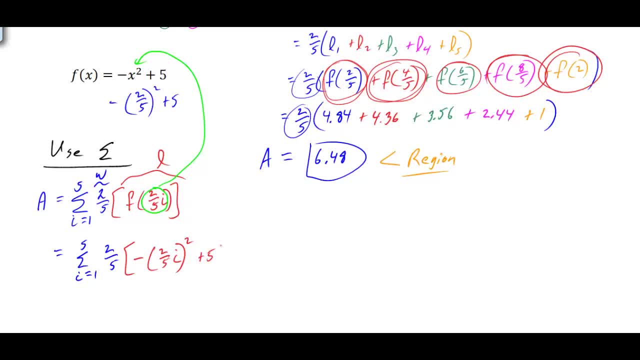 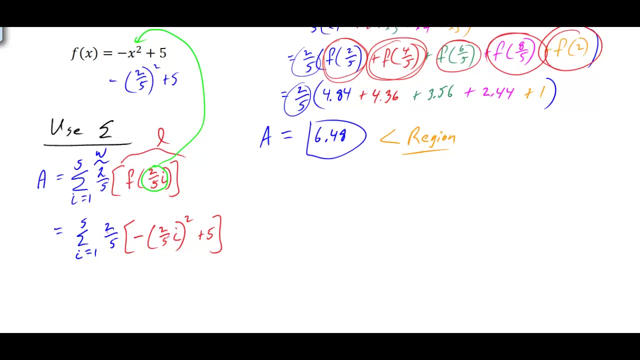 is squared plus 5.. Okay, so now, just like we did in the earlier section here early on in the other videos, we can use your calculator to plug this summation and evaluate this using the calculator. Now, keep in mind here the two-fifths here, because this is a constant. 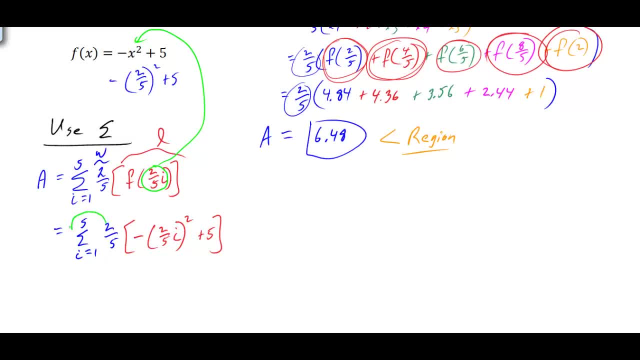 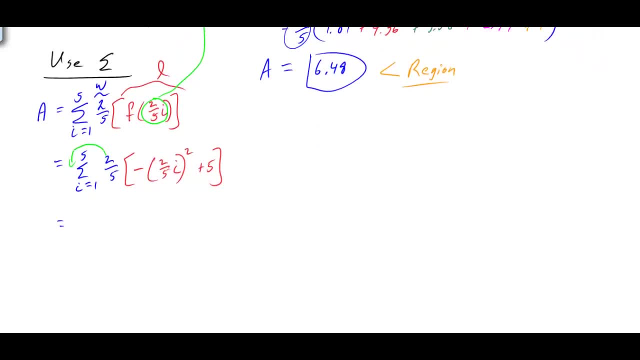 If you wanted to, you could actually take this two-fifths and we could just move that out front, so that you would end up with the sum of i equals 1 to 5. And the two-fifths is out front, And then on the calculator you could just simply type in this: minus two-fifths, i squared.